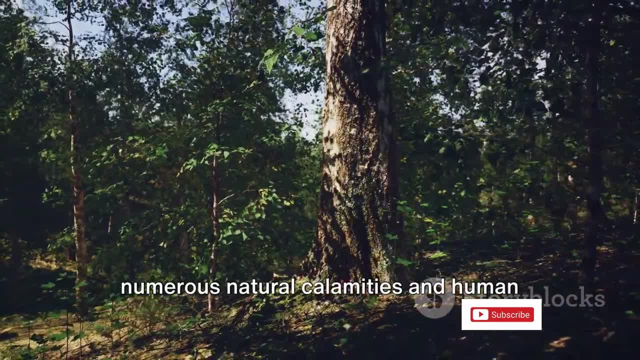 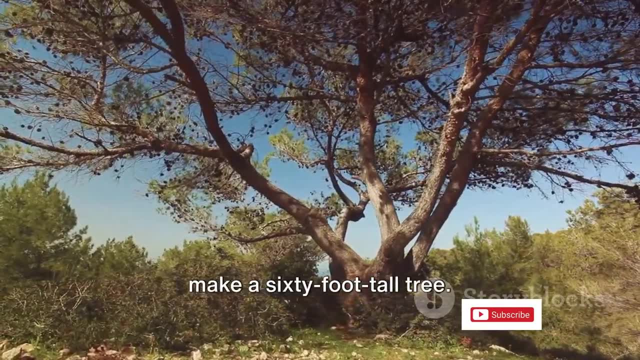 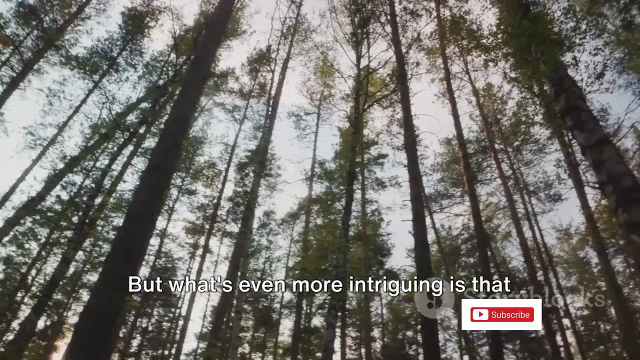 is that, despite facing numerous natural calamities and human interventions, General Sherman continues to grow, adding enough wood each year to make a 60-foot-tall tree. It's not just a tree, It's a testament to nature's resilience and enduring beauty. But what's even? 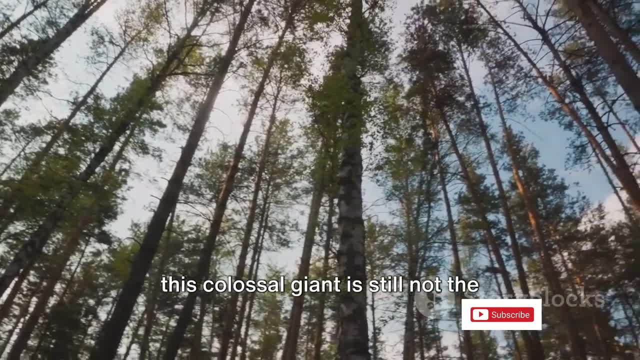 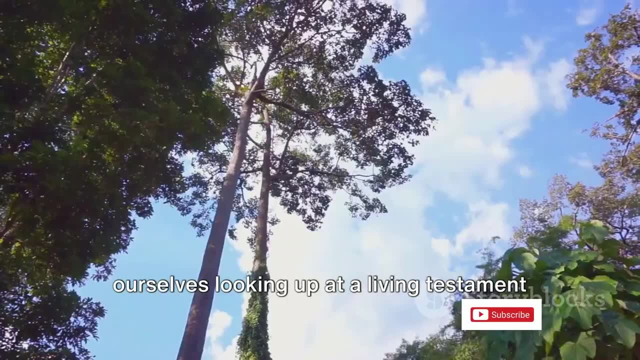 more intriguing is that this colossal giant is still not the biggest tree on our list. An impressive start to our list, wouldn't you say. Moving on to number 9, we find ourselves looking up at a living testament to nature's grandeur. Picture this, A towering giant reaching towards. 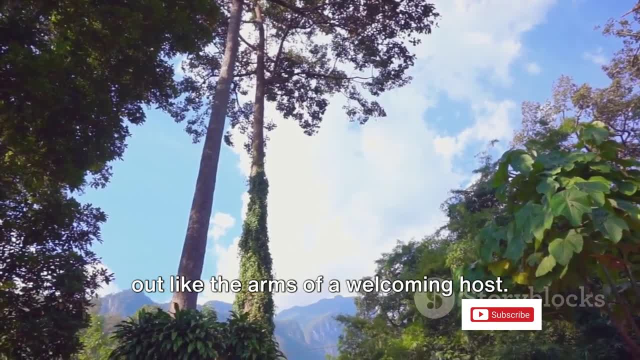 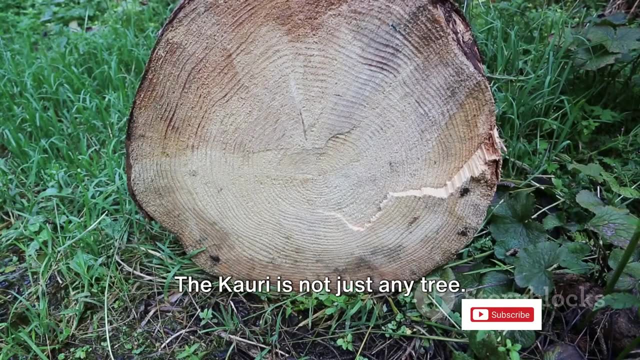 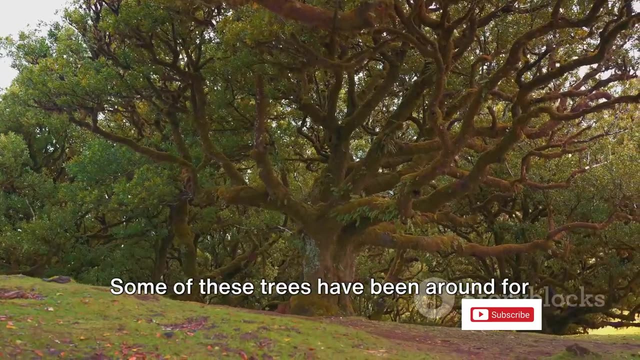 the sky, its branches spreading out like the arms of a welcoming host. This tree, my friends, is the majestic kauri of New Zealand. Now let's delve a little deeper. The kauri is not just any tree. It's one of the most ancient species on earth. Some of these trees have been around for. 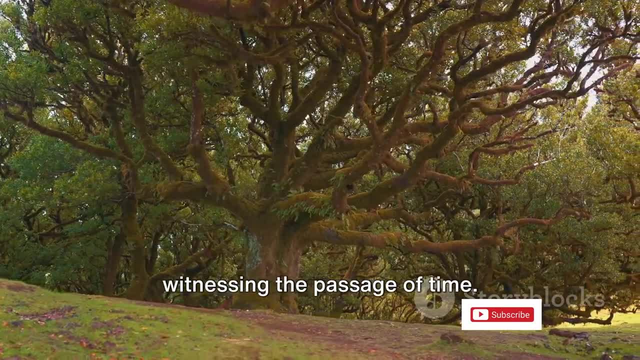 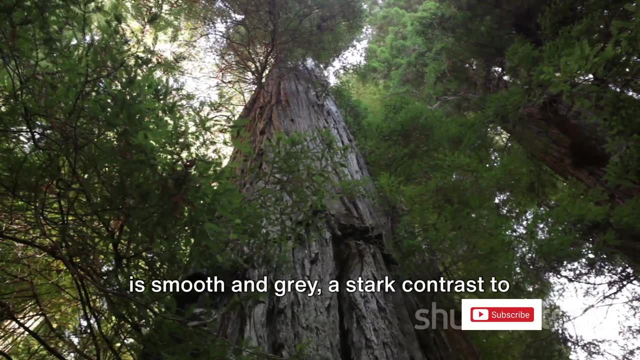 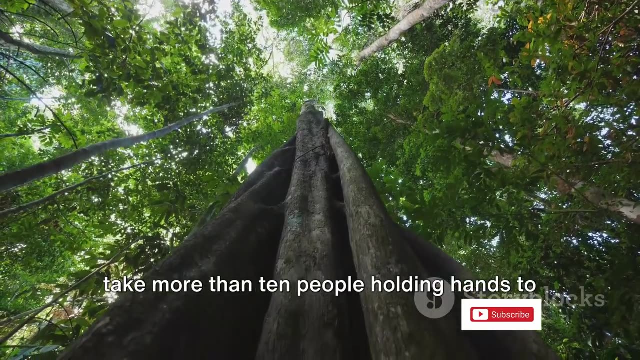 over 2,000 years silently witnessing the passage of time. Imagine if these trees could talk, the stories they would tell. The kauri's bark is smooth and gray, a stark contrast to the deep green of its leaves, And the trunk it's so wide it would take more than 10 people holding hands. 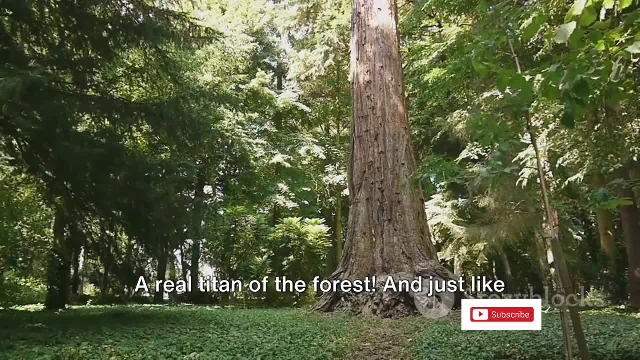 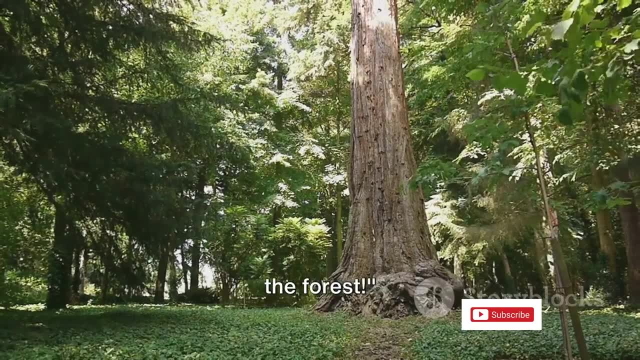 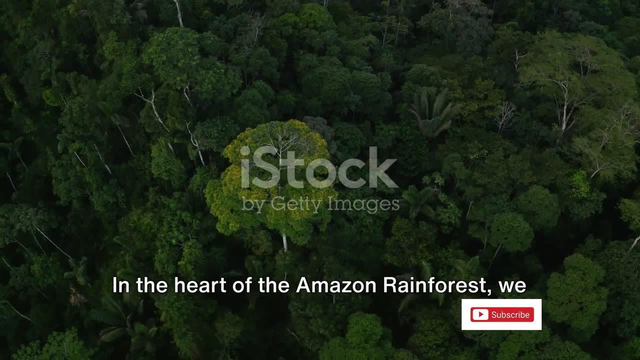 to encircle it, A real titan of the forest. And just like that, we've uncovered the secrets of the ninth largest tree in the world. Now, that's a tree that stands out from the forest At number 8 and 7, we have two trees that are truly remarkable In the heart of the Amazon rainforest. 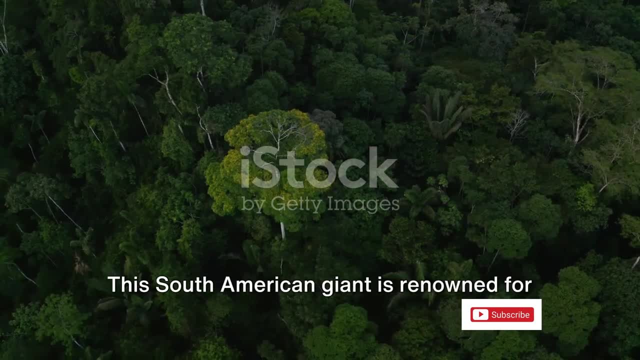 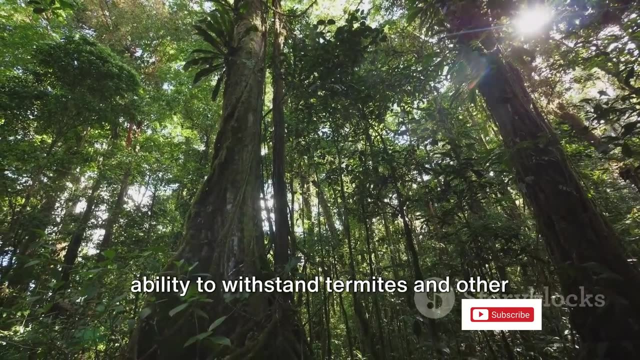 we find our number 8, the Angelum vermello. This South American giant is renowned for its towering height and robust trunk. The Angelum vermello is unique in its ability to withstand termites and other pests, making it a symbol of resilience in the midst of adversity. 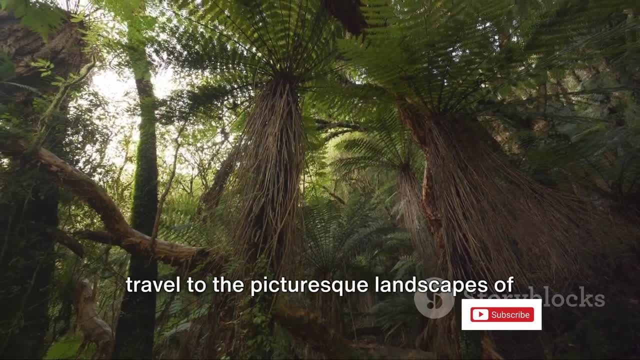 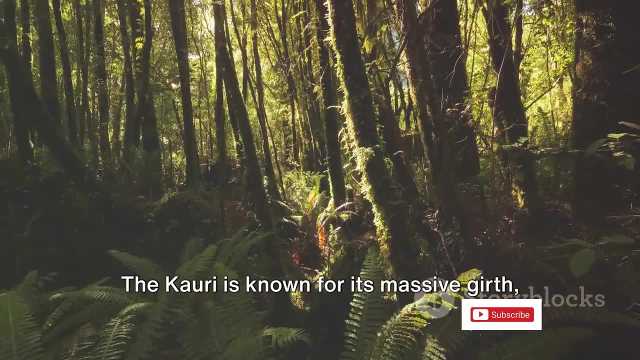 Swiftly moving on to our number 7, we travel to the picturesque landscapes of New Zealand. Here we find the kauri tree, a majestic sight to behold. The kauri is known for its massive girth, some reaching up to 40 feet in diameter. What's more, these trees can live for over 2,000 years. 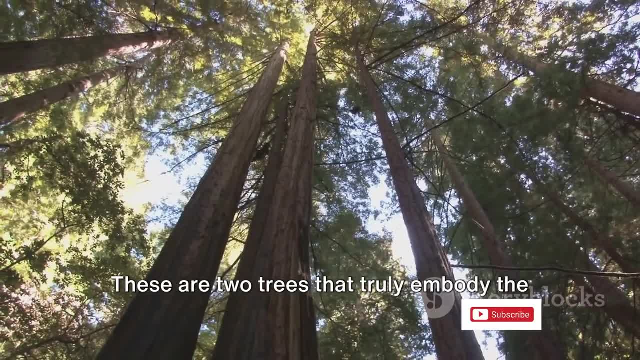 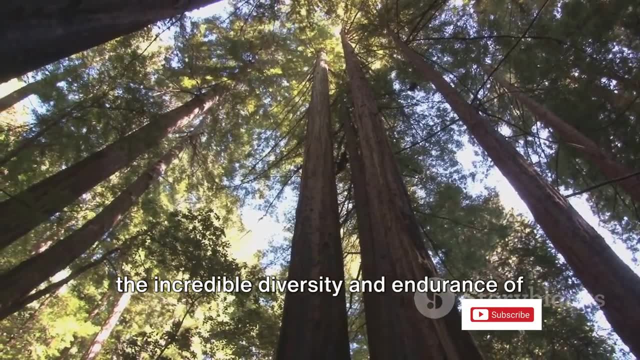 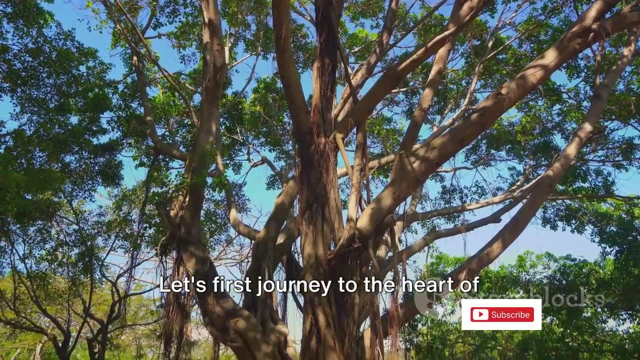 bearing silent widths. These are two trees that truly embody the phrase standing tall. Each in its own way, they remind us of the incredible diversity and endurance of the natural world. Our countdown continues with the sixth and fifth largest trees in the world. Let's first journey to the heart. 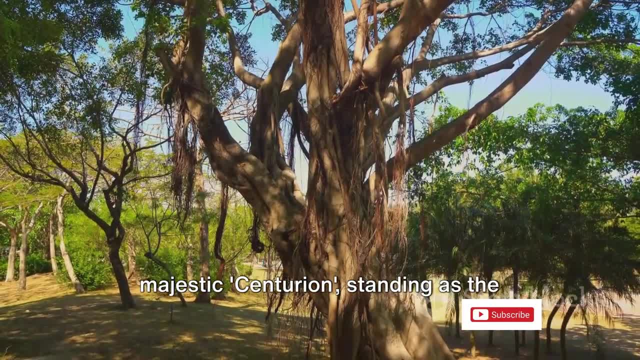 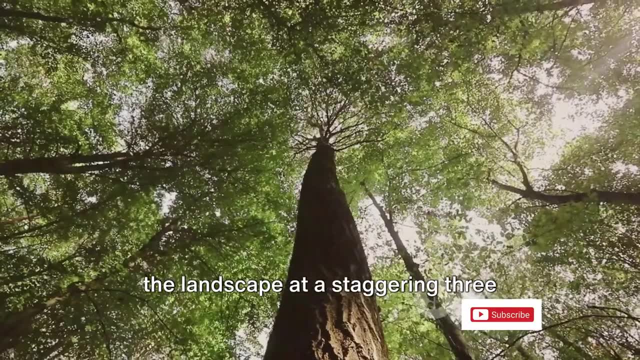 of Queensland, Australia, where we find the majestic centurion standing as the sixth largest tree. This magnificent mountain ash towers over the landscape. at a staggering 329% of its size, The kauri tree is the largest tree in the world. The kauri tree is the largest tree in the 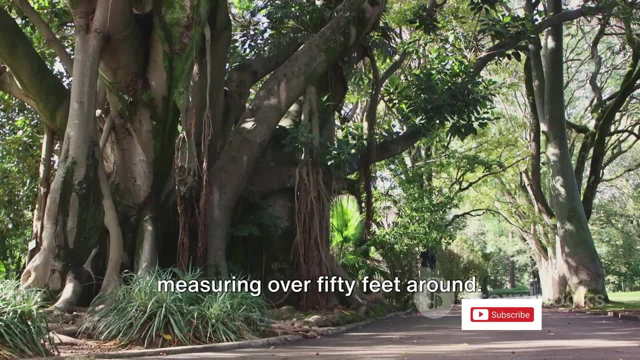 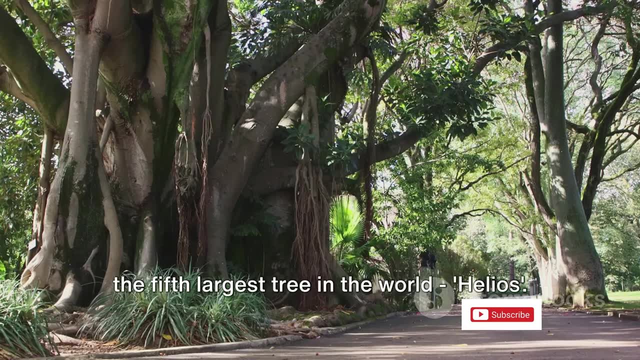 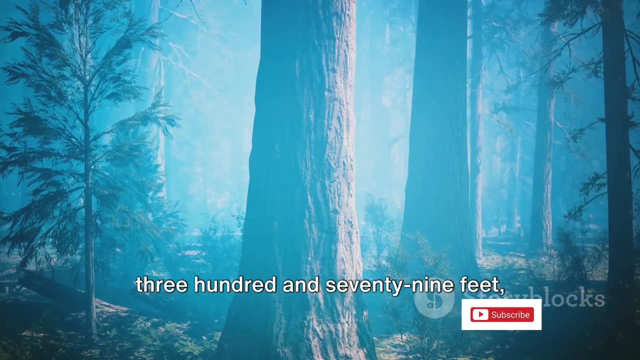 world. Its girth is equally impressive, measuring over 50 feet around. Moving on, we find ourselves in the Redwood National Park, California, home to the fifth largest tree in the world, Helios. This colossal coast redwood reaches up to 379 feet, dwarfing everything. 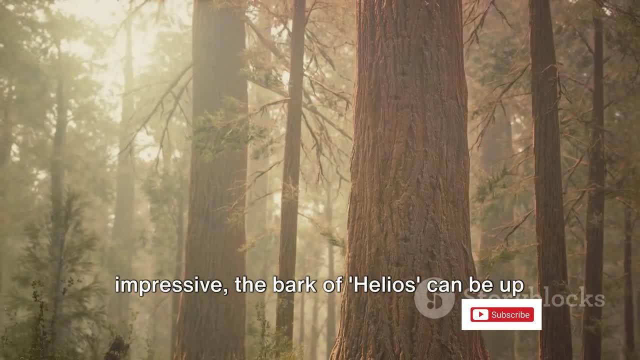 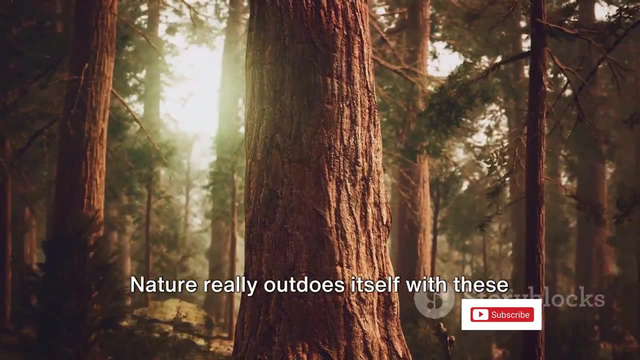 in its vicinity. It's not just the height that's impressive: The bark of Helios can be up to 12 feet thick, providing it with a unique defense mechanism against forest fires. Nature really outdoes itself with these magnificent creations, doesn't it? 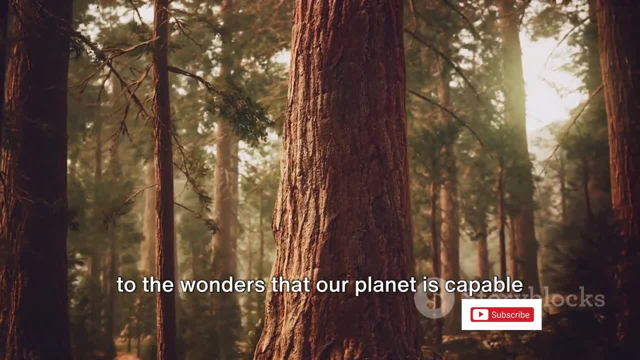 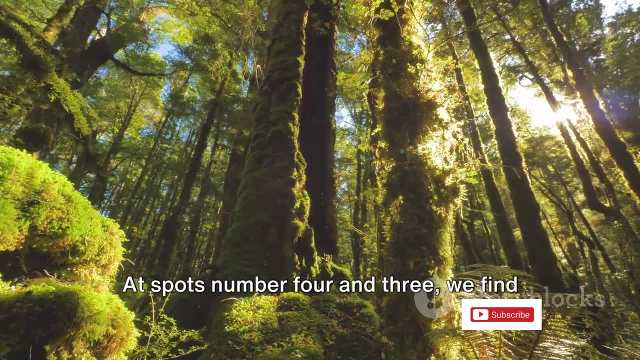 The sheer scale of these trees is a testament to the wonders that our planet is capable of producing. As we climb higher on our list, the trees get even more astounding. At spots number four and three, we find two awe-inspiring giants. In the fourth spot, we encounter the majestic. 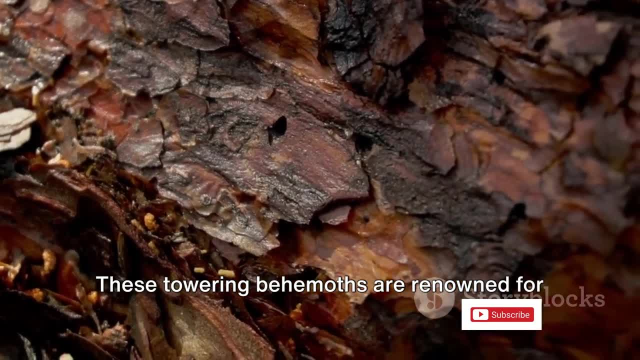 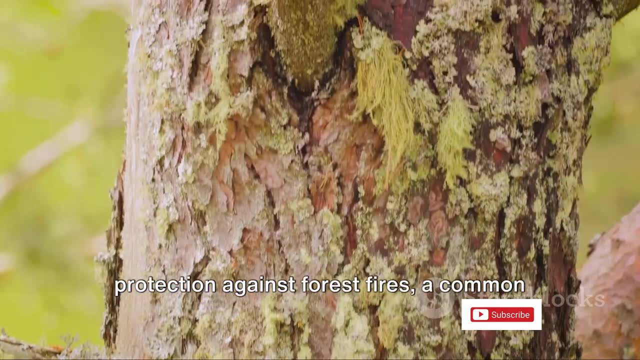 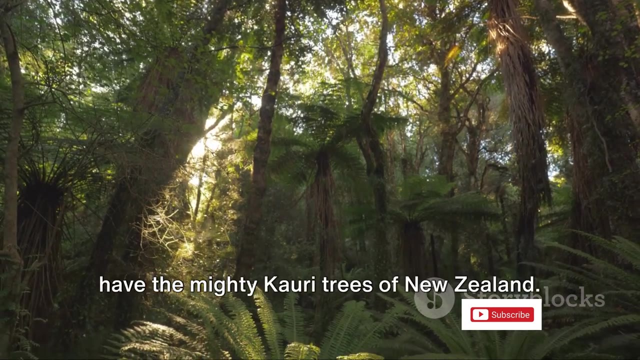 Douglas firs of North America. These towering behemoths are renowned for their height, often reaching up to 300 feet. Their bark is thick and corky, providing protection against forest fires, a common threat in their native regions. Just a notch above, at number three, we have the mighty kauri trees of New Zealand. These 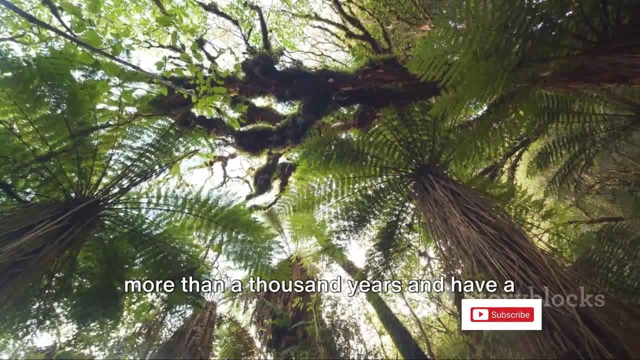 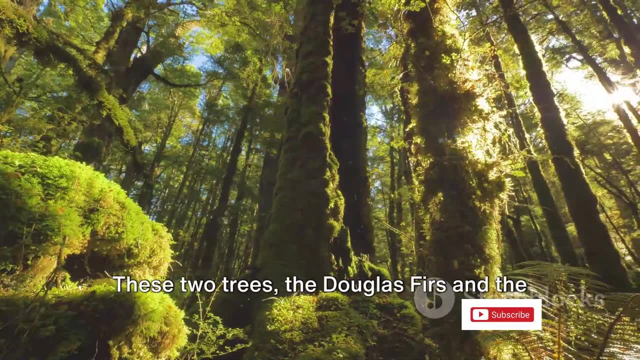 ancient trees have been around for more than a thousand years and have a girth that can reach up to 40 feet. They are truly a sight to behold with their massive trunks and sprawling branches. These two trees, the Douglas firs and the kauris, not only dominate their landscapes, 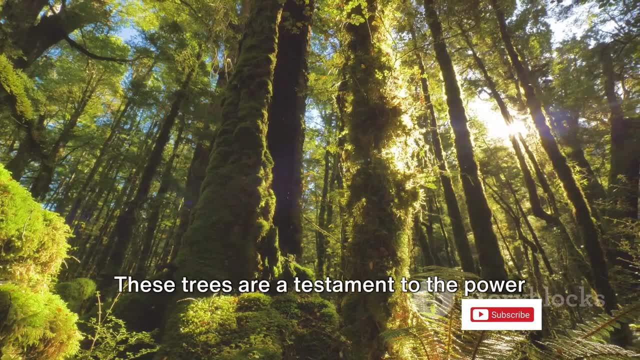 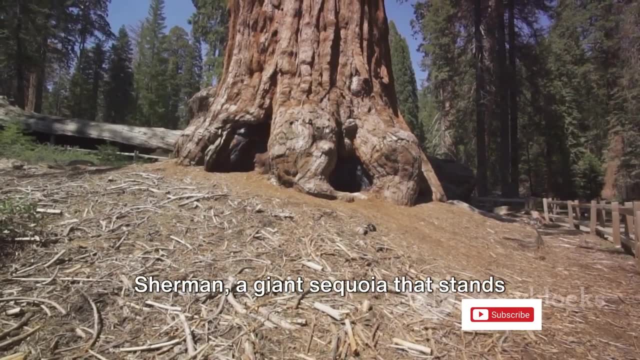 but also our imaginations. with their grandeur, These trees are also known for their unique beauty and power. These trees are a testament to the power and beauty of nature. Just missing out on the top spot, at number two, we have the majestic General Sherman. 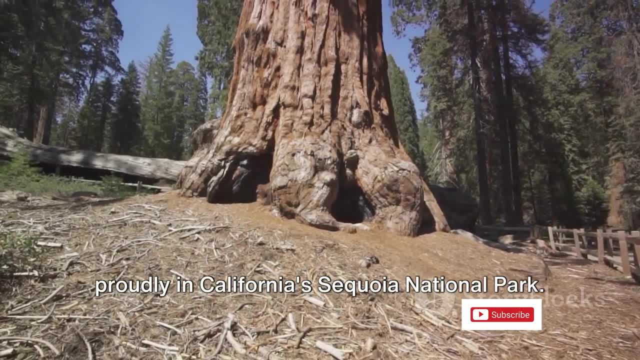 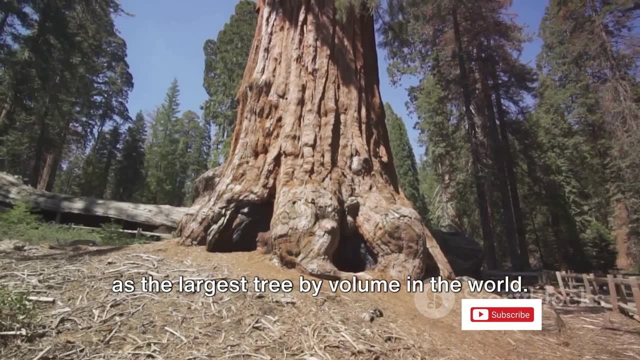 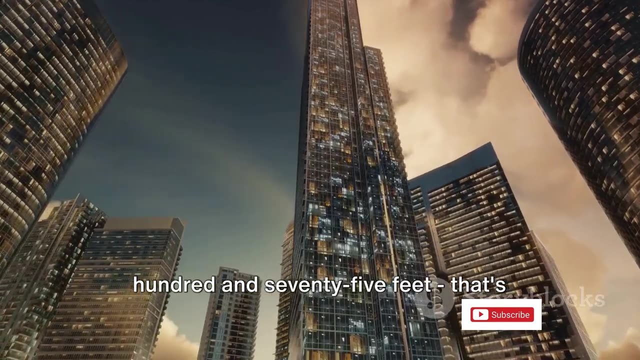 a giant sequoia that stands proudly in California's Sequoia National Park. This titan of nature is not just tall but incredibly bulky. holding the record as the largest tree by volume in the world. Its impressive stature is a sight to behold, reaching a height of nearly 275 feet. That's. 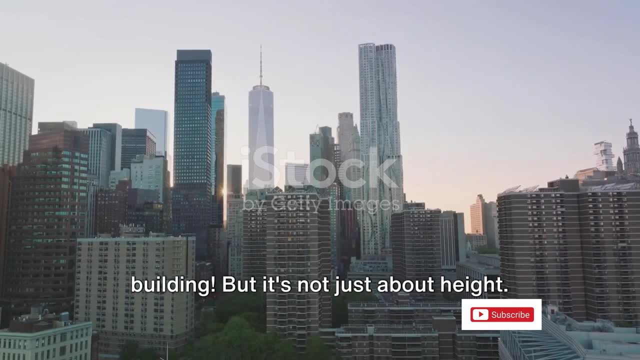 about as tall as a 27-story building. The largest tree in the world is a giant sequoia, which stands proudly in California's Sequoia National Park. But it's not just about height: This tree's girth is equally impressive, boasting an astounding 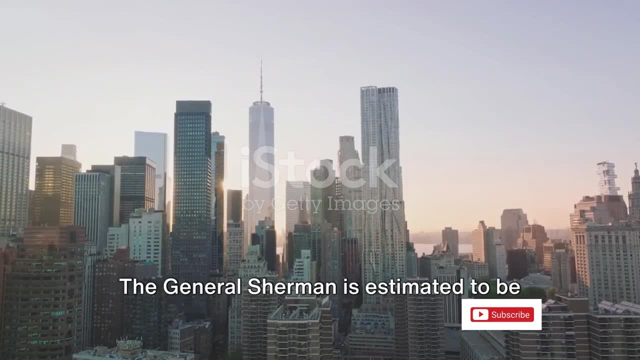 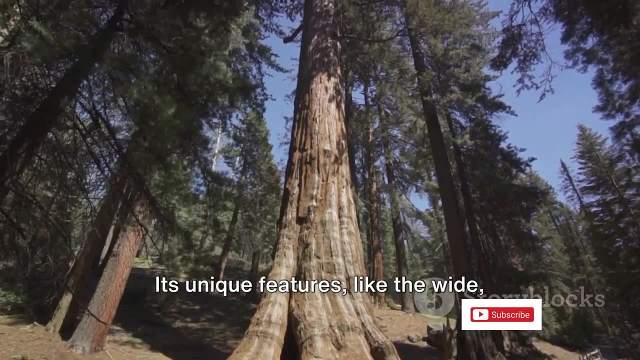 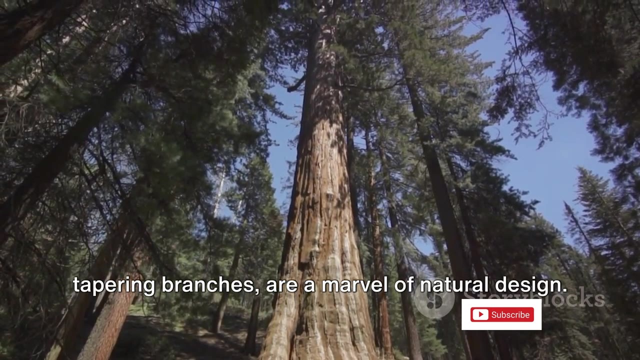 diameter of nearly 36 feet at its base. The General Sherman is estimated to be over 2,000 years old, a living testament to the enduring power of nature. Its unique features, like the wide fire-resistant bark and the lofty tapering branches, are a marvel of natural. 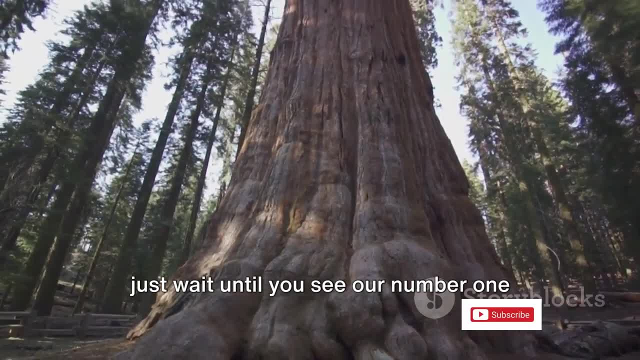 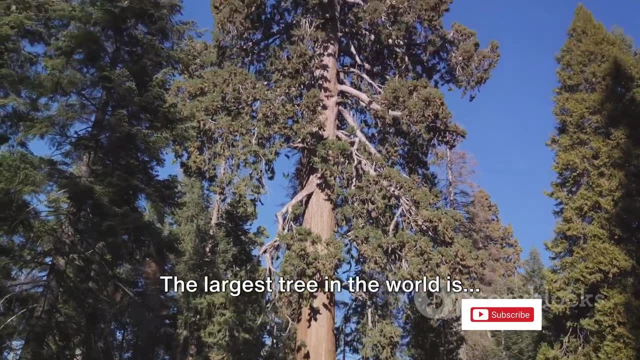 design, A close contender for the top spot. but just wait until you see our video, Wait until you see our number one tree. And finally, the moment we've all been waiting for: The largest tree in the world is the General Sherman tree. 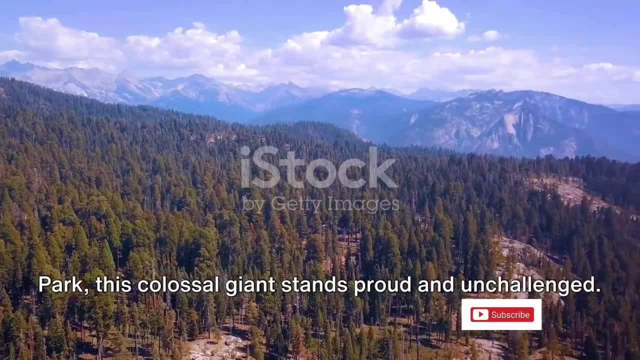 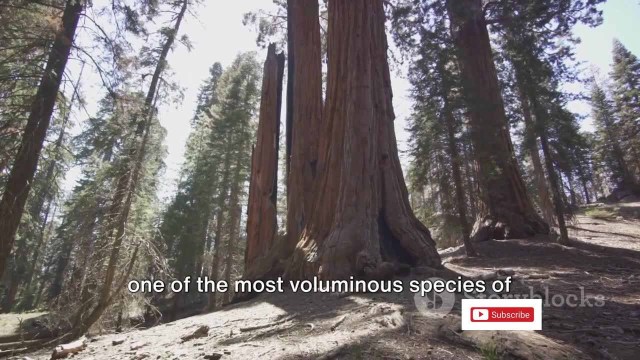 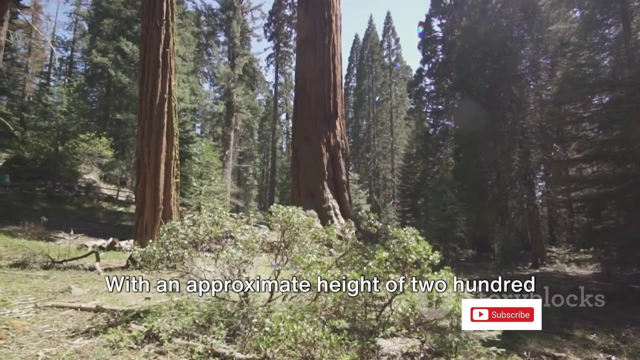 Nestled within the heart of California's Sequoia National Park, this colossal giant stands proud and unchallenged. The General Sherman is a sequoia tree, one of the most voluminous species of trees on the planet, But what sets it apart is its staggering dimensions, With an approximate height of 275 feet and 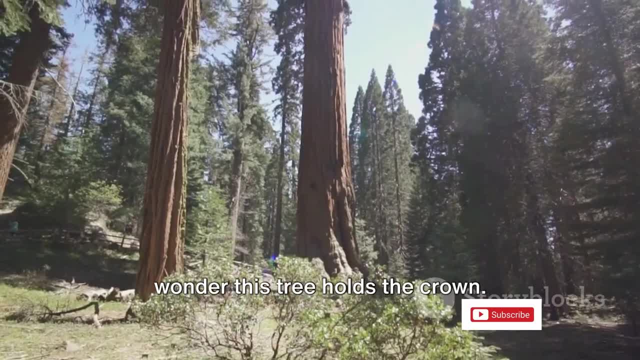 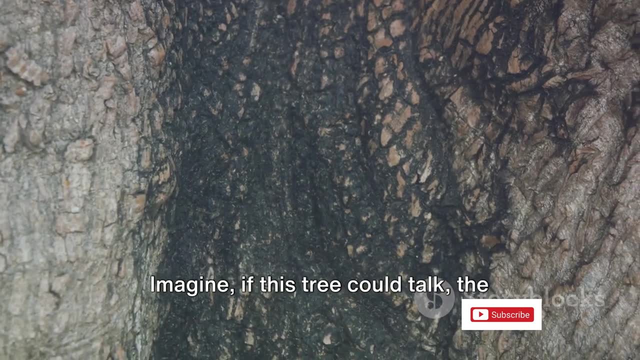 a diameter of 25 feet at its base. it's no wonder this tree holds the crown. Its age, estimated to be over 2,000 years, adds to its majesty. Imagine if this tree could talk, the stories it could tell. 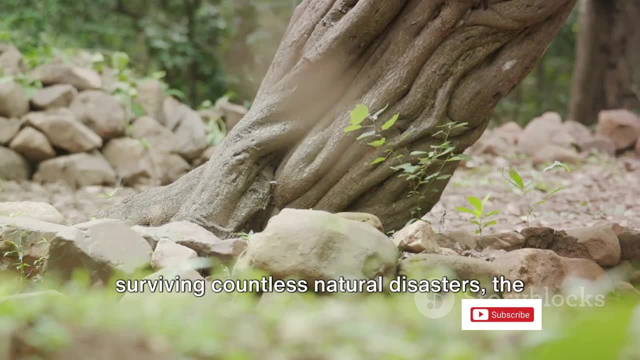 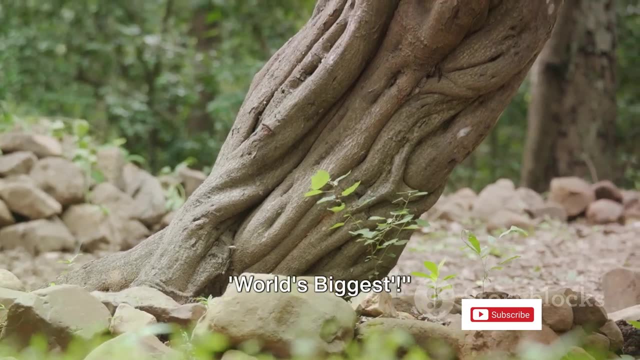 From witnessing the rise and fall of civilizations to surviving countless natural disasters, the General Sherman stands as a testament to resilience and endurance. Now that's a tree worthy of the title: World's Biggest. And there you have it: the 10 biggest trees in the world. 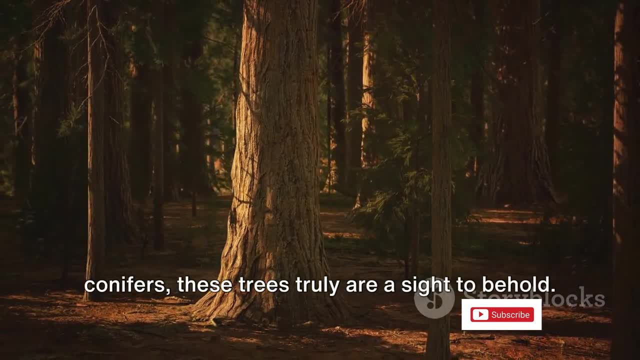 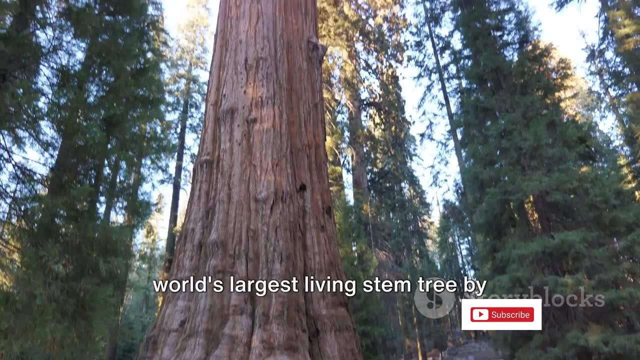 10. The General Sherman Tree. From titans to colossal conifers, these trees truly are a sight to behold. We've journeyed from the expansive branches of the General Sherman, the world's largest living stem tree by volume, to the massive girth of the Sunland Baobab, a tree with a 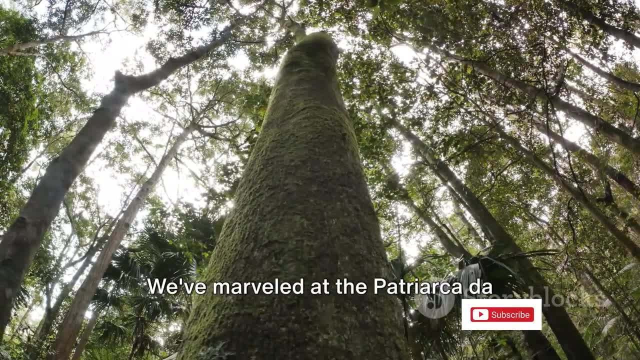 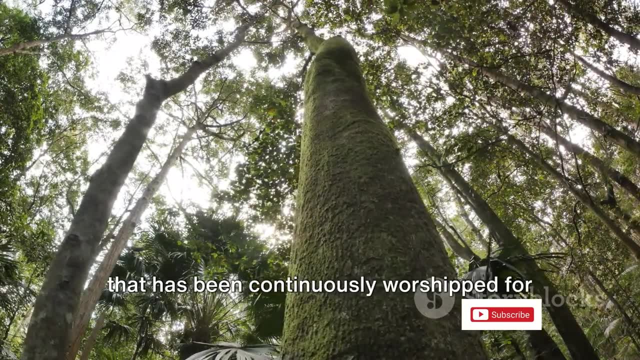 pub. inside its trunk, We've marveled at the Patriarca da Floresta, a towering Brazilian hardwood, and the sacred Sri Mahabodhi, a fig tree that has been continuously worshipped for over 2,000 years. 10..